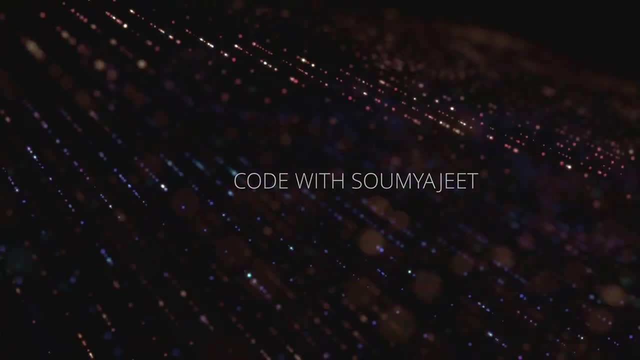 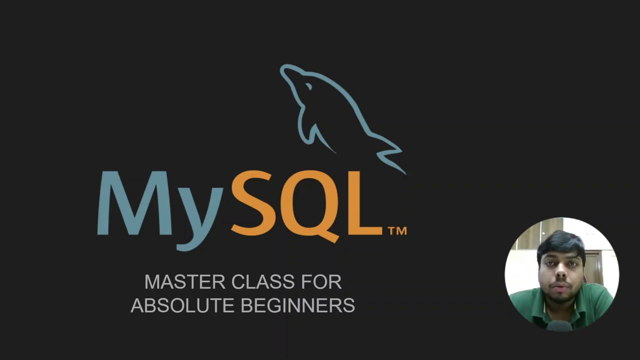 Hello friends, I want to welcome you to my course on MySQL database. So I have made this course for developers who want to learn about MySQL database and those who want to work on backend. learning of database and database management system is very important, So this course is catered for them. 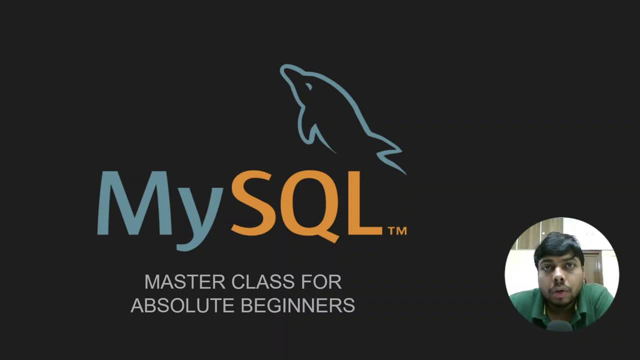 So if you are looking for a course on database certification or database administration or data analysis, then probably this course is not right for you. This course is specifically designed for developers, Because I myself am a developer and I have developed this course by putting all my 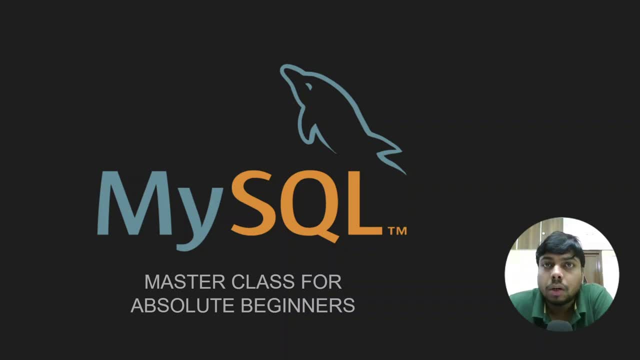 learning all my experience, all my ups and downs that I have endured during my nine years of experience in this software realm Right. So I hope this course will help you Right. This course is specifically on MySQL database or relational database. This course does not target the NoSQL database, like MongoDB and those kind of stuff. This is pure. 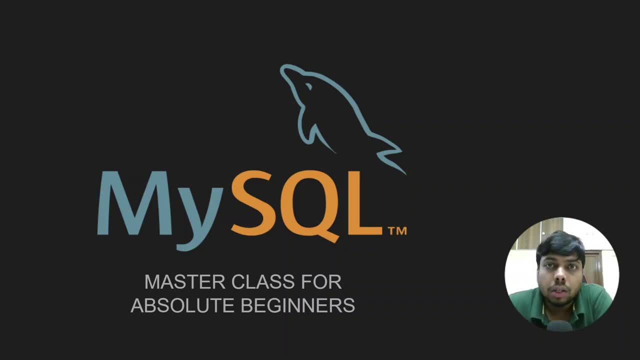 relational database, Right. So whatever you learn, these are relational database concepts. I have taken MySQL here as an example. Now, the learning of database is extremely important. Right, It is the backbone of any software company, or any company for that matter. Right, They say data is the new oil. 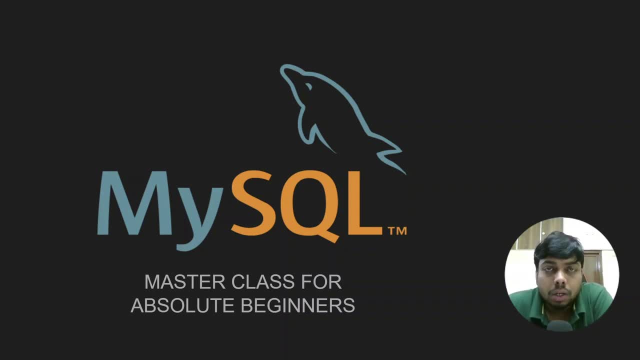 Right. If you don't have understanding about how database internally works- right, how to write queries, how to create or organize your data, its schema, then it's very difficult to survive in software industry. Right, It's very crucial for you to understand the database, its management system, right, and all the concept that is. 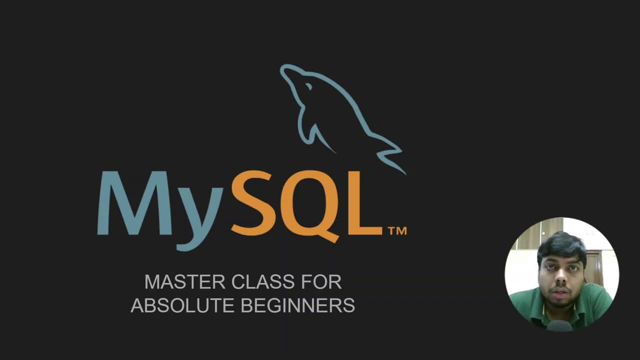 the database. right, that's what makes a seasoned software engineer. specifically, you know a back-end software engineer, right? if you are looking to go into back-end software development, then understanding of database is extremely important, right? so this is what the course is designed for. we will start from absolute zero, as if you are a beginner, and slowly, slowly, we'll keep on taking. 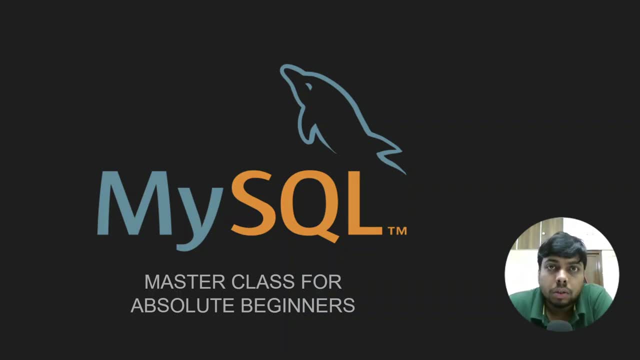 up a notch, up a notch and we'll go towards advanced concept. this course will be mostly hands-on. there are one or two places where i'll be using little bit of powerpoint to explain the concept, but otherwise this course is extremely handsome. i'll be writing the query and i'll be 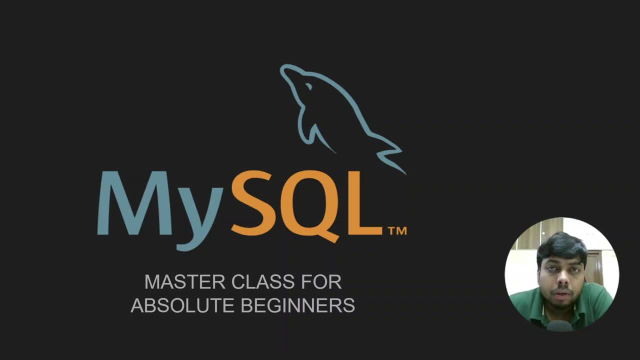 running the query, and i'll give one. i'll give you the live uh example of how the query is written and how its output will be structured. right now, in order to take this course, what you need? of course, you need a mysql database instance right. there are a couple of ways in which you can. 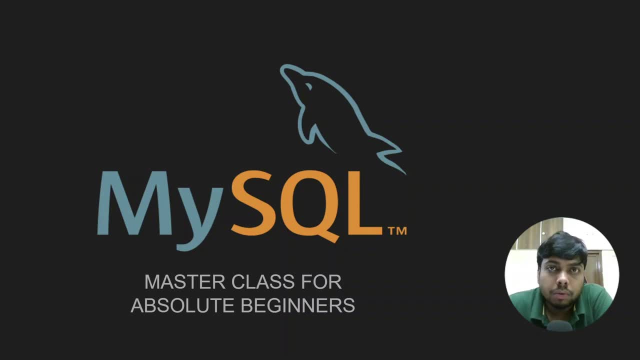 uh, get the database instance. one is using a cloud service provider. right, you can go to any cloud service provider like amazon aws. from there you can take a mysql instance. all you have to do is you should know the url or the host name of the sql database, its port number and its user id, and 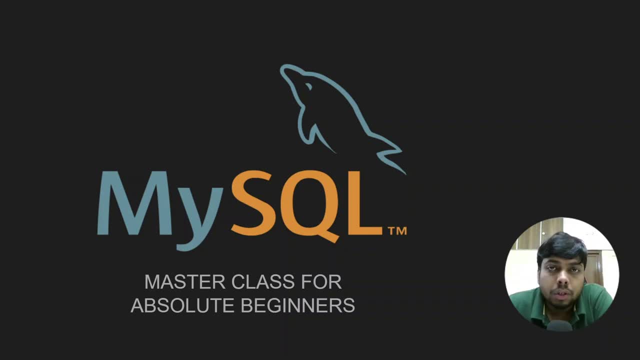 password that you need to connect right. if you have this information at hand, then you can proceed with. alternatively, what you can do is you can install a mysql server engine on your local system, right? it is available for both mac and os. you know operating system if you go to the mysql website. 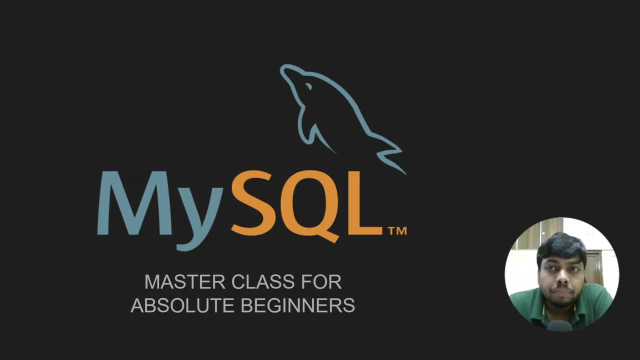 there is a community edition that if you install right, that you should be able to install in your system and with that, uh, it will run as a local host, it will run on a port number and id and password you can configure during installation. and there is another method. 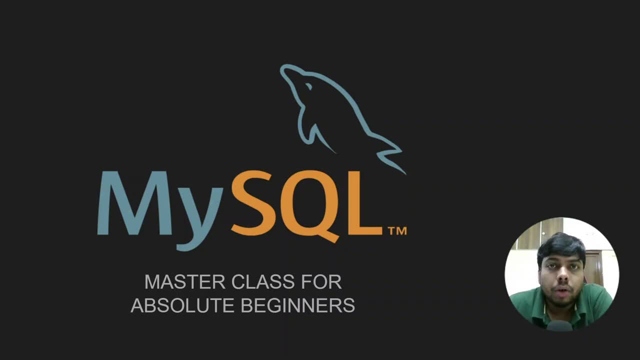 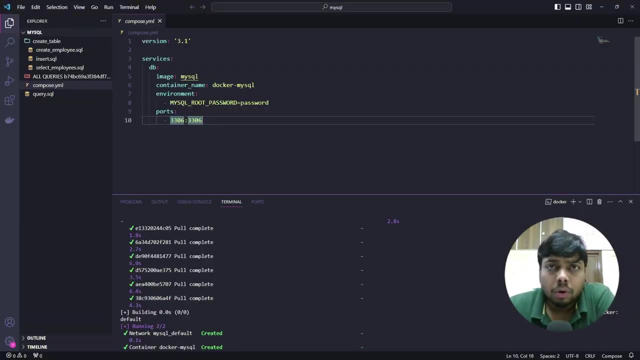 that is using docker right. so what you can do is you can write a docker compose file. i'll show you my docker compose file, right. so if you don't know docker, that's fine. if you know docker, you can see this one. this is a docker compose file. 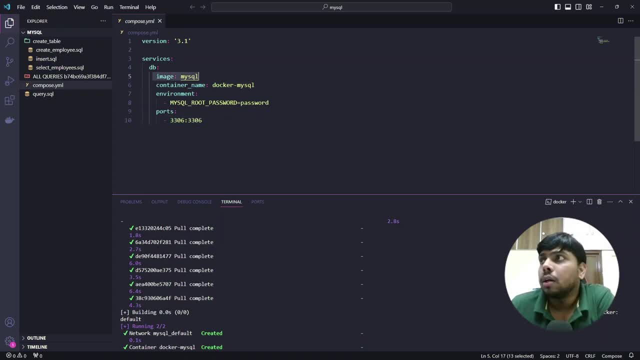 what this will do is. this will take a mysql image right. i have named it as docker mysql, right, and its password is, of course, password. i have kept it, of course. if you want, you can change it right, and by default the docker username will be root, right, and it is running on port 3306. and inside the container and outside the container it is pointing to port same port, 3306. right now. if you run docker, compose up right like how i have done here. you will get a running instance of the docker right. so these are the three options i leave. 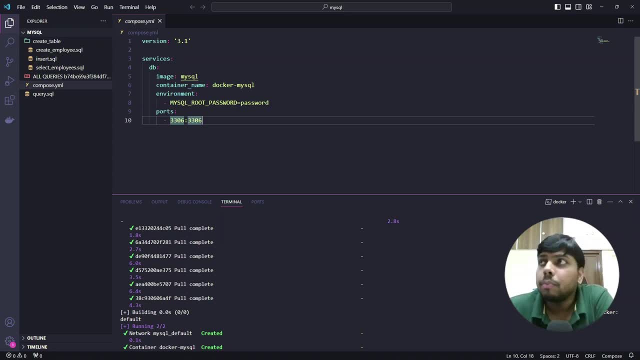 up to you what option you prefer. the best right for me, i am going to use the docker compose because that's what i feel convenient, right? so i'll be using the docker compose method. of course, if you want, you can go for a cloud instance or, if you want, if you feel convenient. 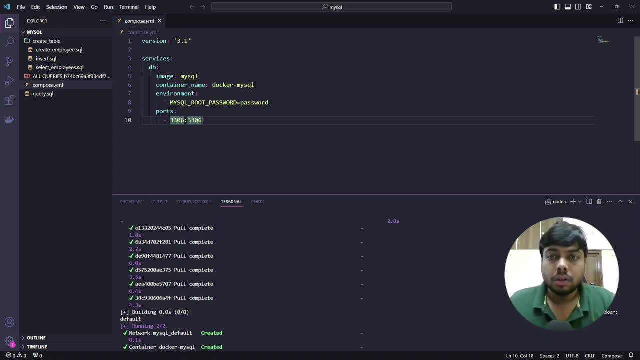 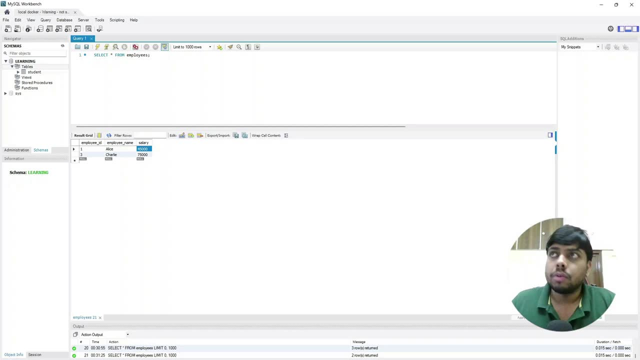 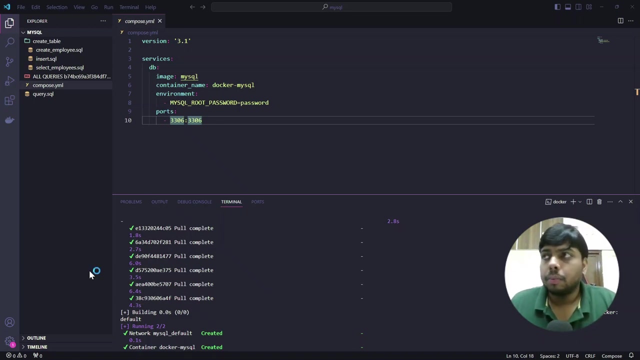 you can install the uh mysql database server instance in your system. now, how to connect to the database, right? so there is a tool called mysql workbench, right? so there is a tool called mysql workbench right? so if you open that tool it will help you connect into the database, right? 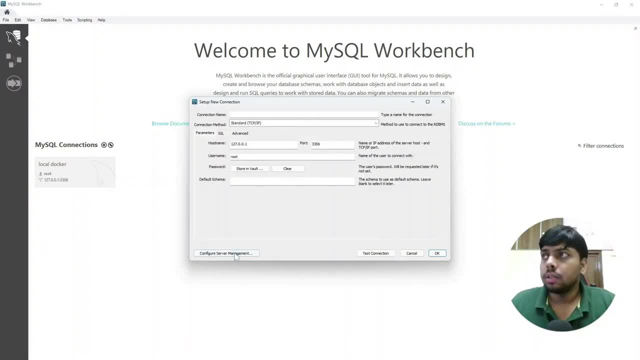 so here what you can do is you can add a new connection right. you can give a connection name you. you can give any name to this one right. here you have to give the host name right. whatever is your host name, for me it is the local host or the loopback ip address for you, if you have taken it. 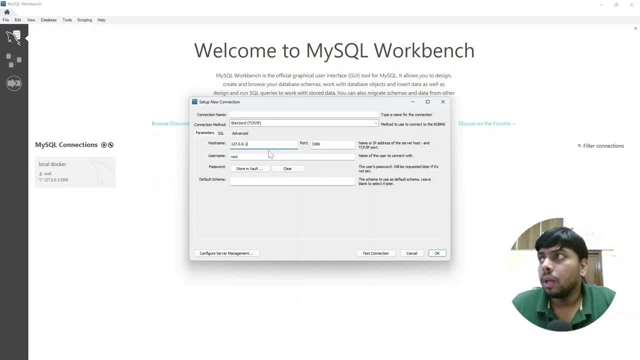 from a you know cloud service provider from their console you can get the host name right. so i am right, this is the port, this is the username root, and you have to give a password, right. with that you should be able to connect. right, you will get this kind of a icon and with that, 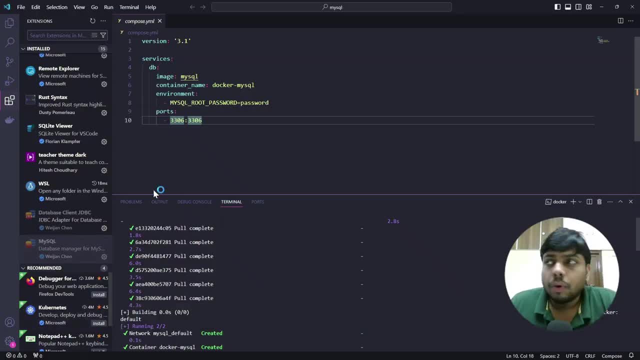 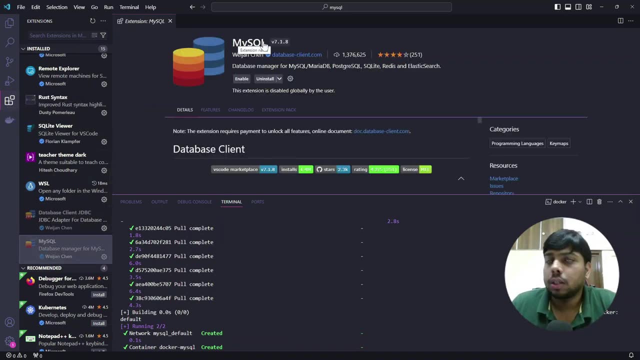 you should be able to connect into the database, right? so for me, what i am going to use is a vs code extension, right? so what this vs code extension is, this is mysql extension, right, so i'll enable this one for you. you might have to do an installation, right. 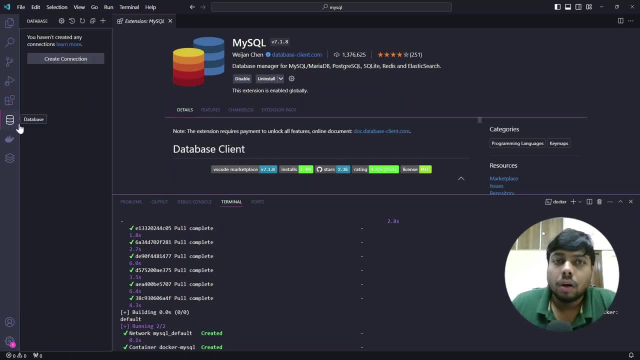 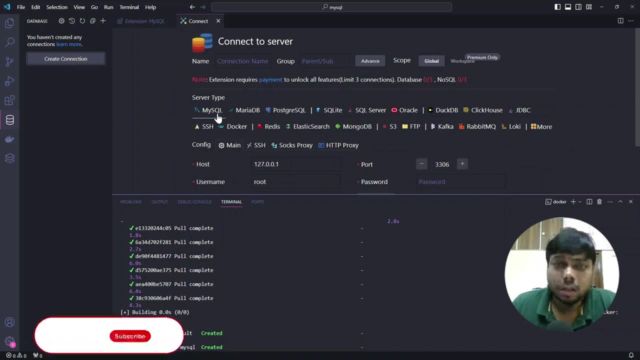 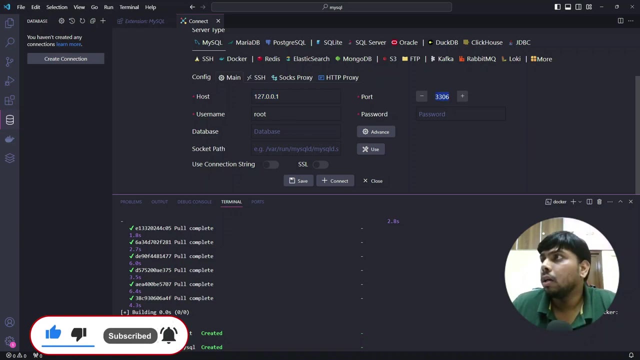 once that is done, you will get this kind of a icon here on your vs code, right? so what you can do is create a connection right. then select the mysql: right here you have to add the host name. here you have to give your port right username and password: right with that. 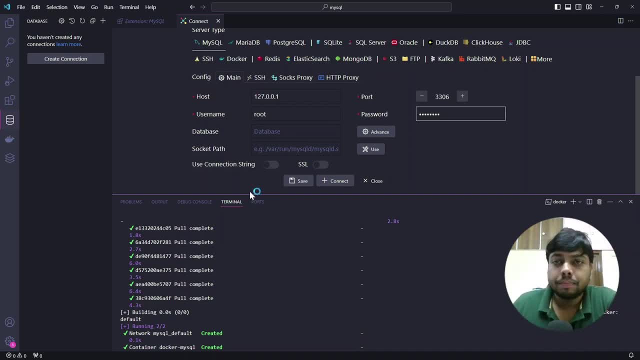 you should be able to connect right. so password right now. what i will do is i'll need to connect right. if you see here it has connected right now. if i scroll down this one, i have some database. so what you can do is i already have a database called learning. if you want, you can create your.